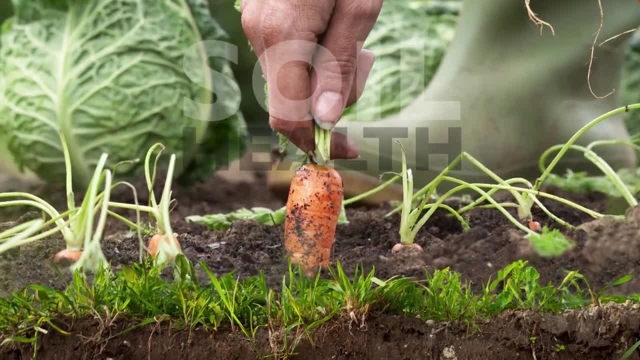 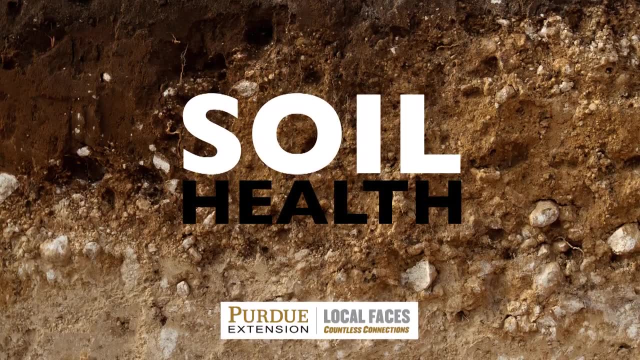 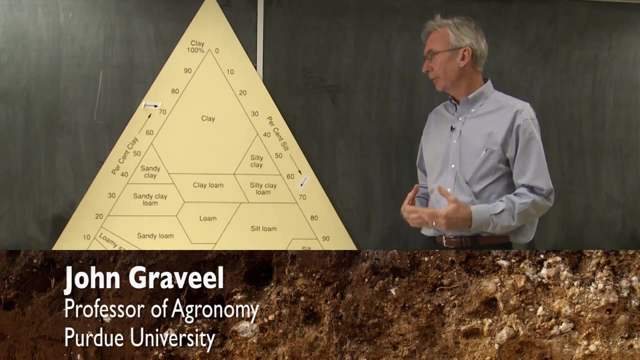 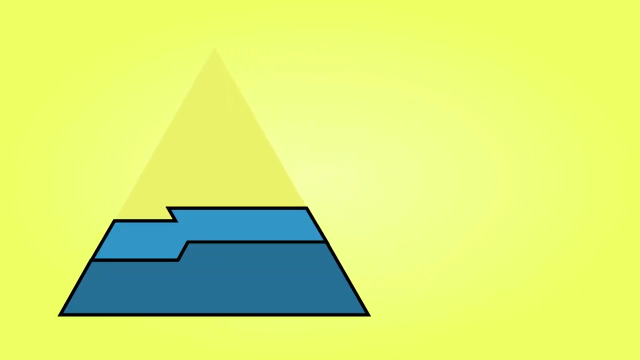 We're going to spend a few moments talking about the textural triangle. Texture is one of those components- the physical properties of soils. that's very important. So the first thing that we like to do with the textural triangle is divide it up into three components. We have 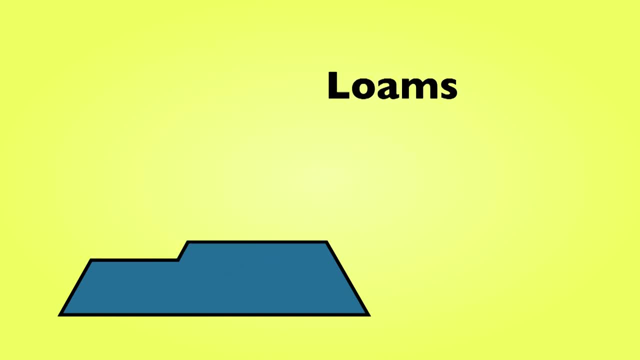 what are called the loams which go from zero up to about 26% clay Loamy, sand sandy loam, loam, silt loam- those are considered. loams From 26% to 40% clay, those are considered. 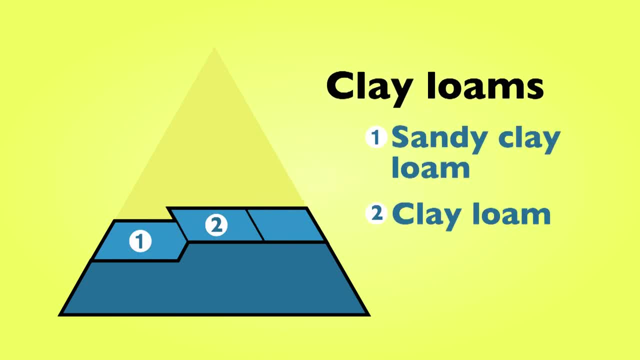 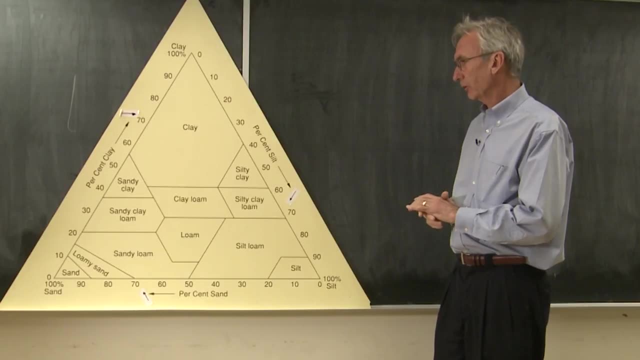 the clay loams: Sandy clay loam, clay loam and silty clay loam. Anything above 40% clay loam, those are considered clays. So sandy clay and silty clay. One thing you want to know about the textural triangle and I usually tell my students in the introductory soils: 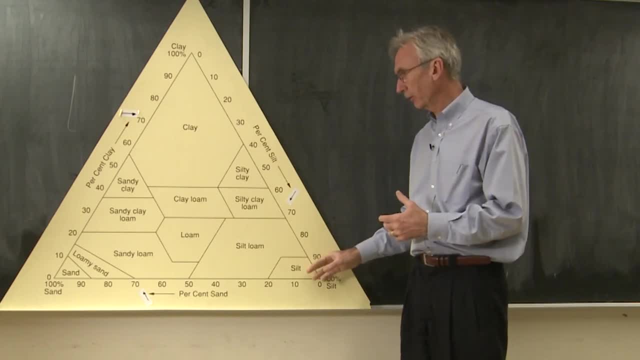 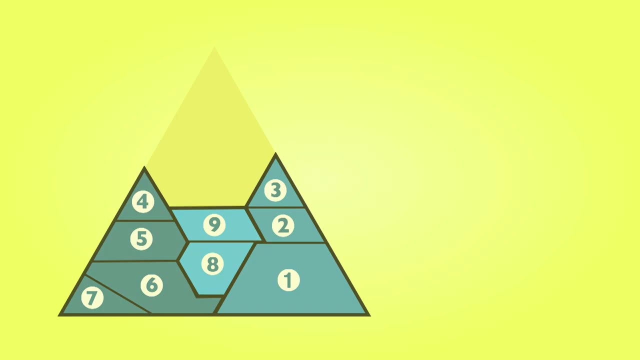 class is that rarely, if ever, you're going to have pure silt or pure sand or pure clay. So actually now you only have really nine textures that you really need to deal with, Those soils which are on the right side of the textural triangle. those are usually soft. 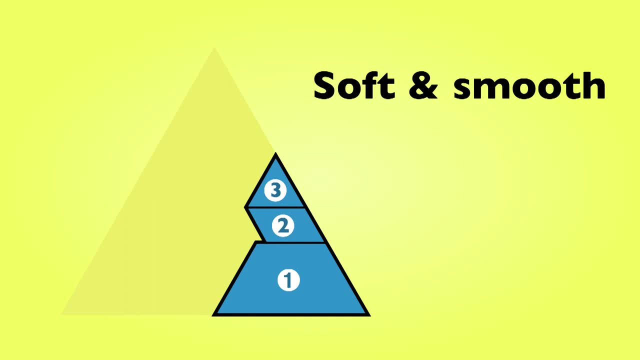 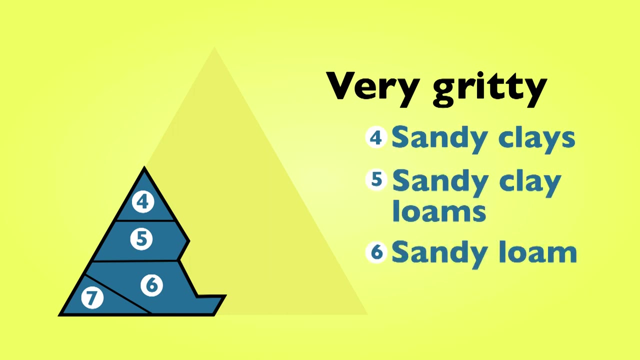 and very smooth. They feel like talcum powder. actually Those are the silts, silt loam, silty clay loam or silty clay. Those soils on the left side of the textural triangle are very gritty in texture. They're sandy clay, sandy clay loam, sandy loam and loamy sand. Now 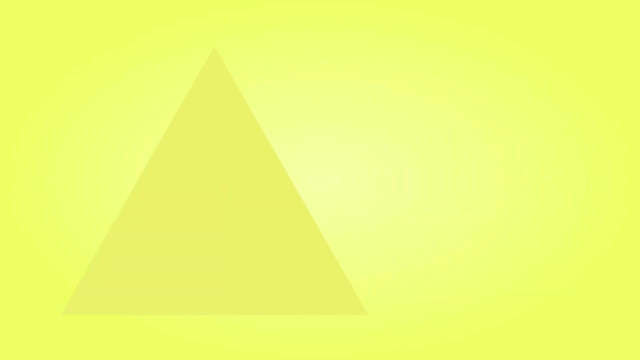 if you're texturing a soil and you don't have a lot of texture, you're going to have a lot of texture. You can't quite figure out exactly. It doesn't feel smooth and it doesn't feel real gritty. Well, that means you're right. smack in the middle of the textural triangle. 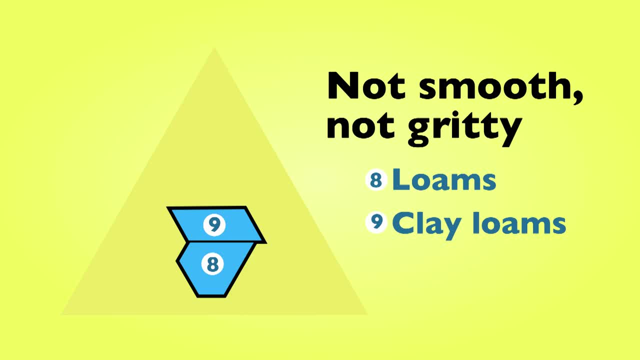 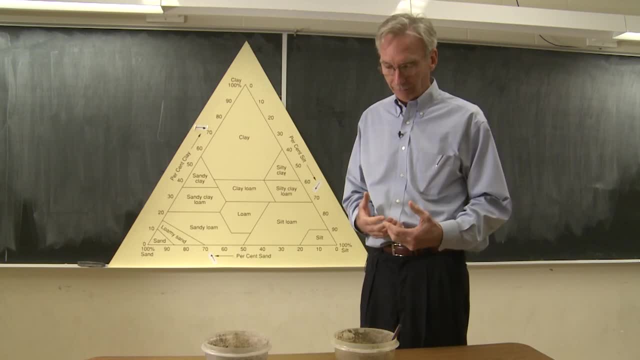 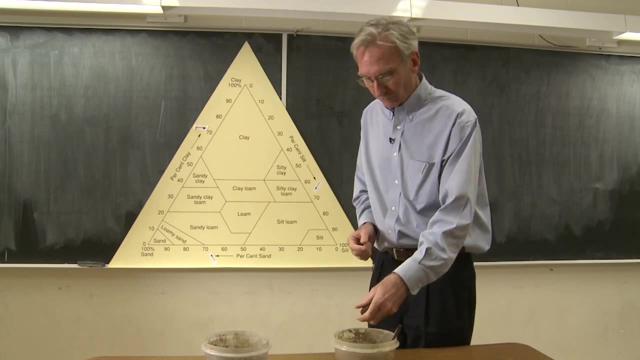 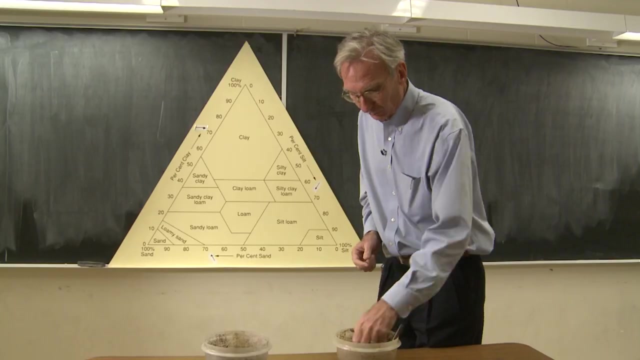 Those are going to be the loams and the clay loams. So let's go ahead and texture a couple of samples and I'll show you how to go about actually doing a soil texture. The first key thing about texturing a soil Is to make sure you've got enough material in your hand, enough soil, I would say have.